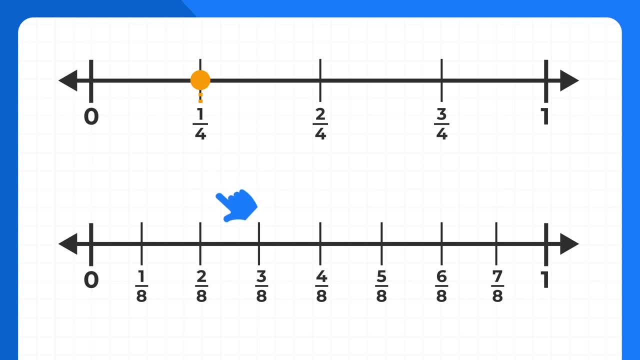 we look at one fourth, we could trace down and see that it's at the exact same place as two eighths. One-fourths and two eighths are equivalent. If you shaded one fourth and you shaded two eights, you can see it's the same amount. So the first equivalent fraction is that one. 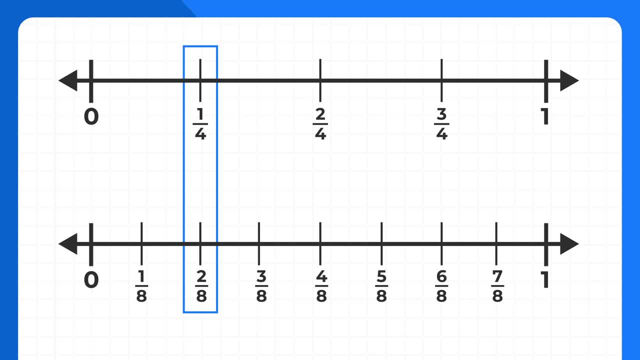 fourth is equal to two eighths. Now, there are other equivalent fractions on this number line too. If we look at two fourths, we can trace it down to the bottom and see that it's equivalent to four eighths. Finally, we could look at three fourths—we could. 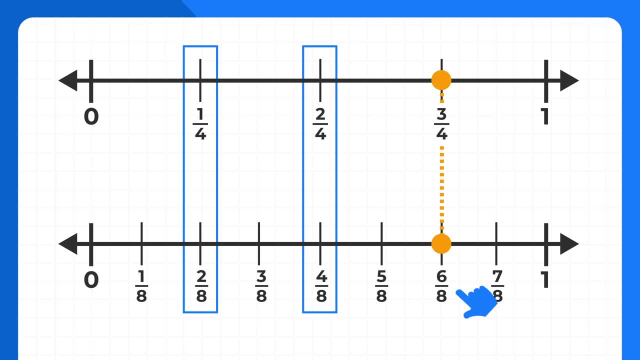 trace it to the bottom and see that it's equivalent to four eighths. Finally, we could down and find 6 8ths, 3 4ths and 6 8ths are equivalent. So on a number line, just look. 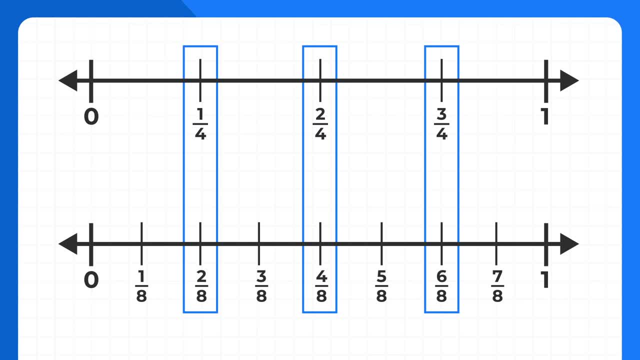 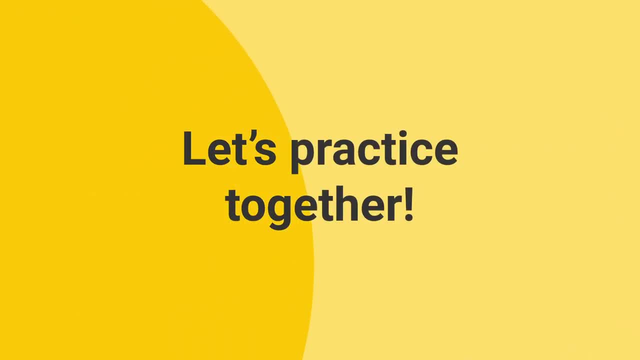 for fractions that are in the exact same place and those will be equivalent fractions. So now that you've seen how to find equivalent fractions on a number line, let's do some practice together. Let's identify any equivalent fractions from these two number lines. Remember. 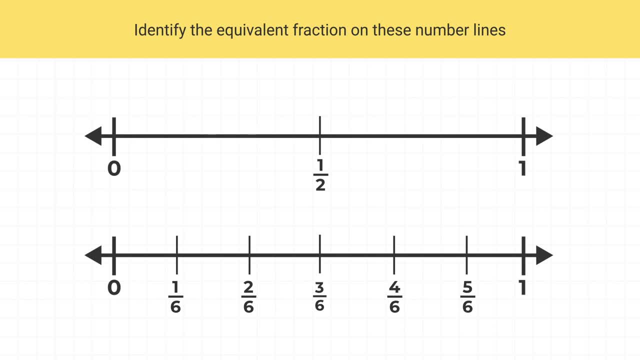 that equivalent fractions are at the exact same place on their number lines. 1 half is at the exact same spot as what fraction We can see 1 half is at the same spot as 3- 6ths. so we can say 1 half is equal to 3- 6ths. Here's another problem to practice with What equivalent? 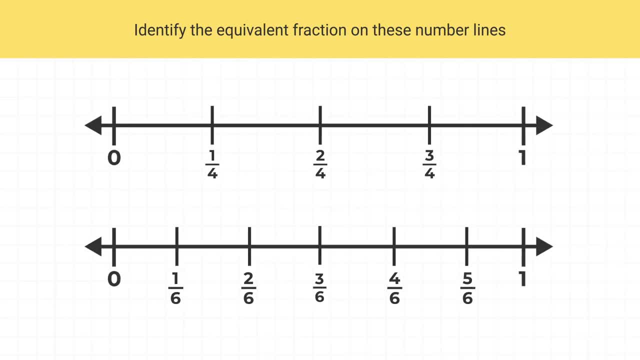 fractions can we identify on these two number lines? Well, let's start by looking at 1- 4th. What fractions are at the exact same spot as 1- 4th? If you trace your finger down, you can see that no fraction is at the exact same spot. 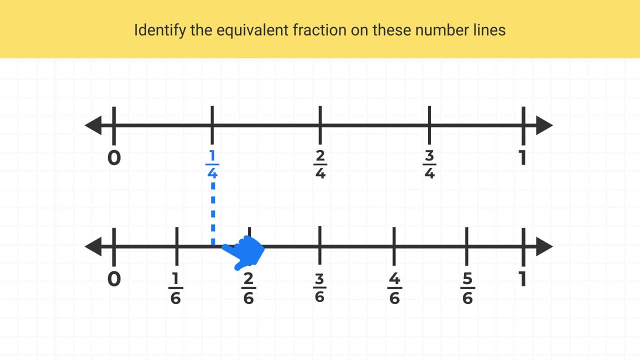 as one-fourth, So no fraction on these number lines is equivalent to one-fourth. What about two-fourths, though? What fraction is at the same place as two-fourths? We can see that three-sixths is at the same spot as two-fourths. 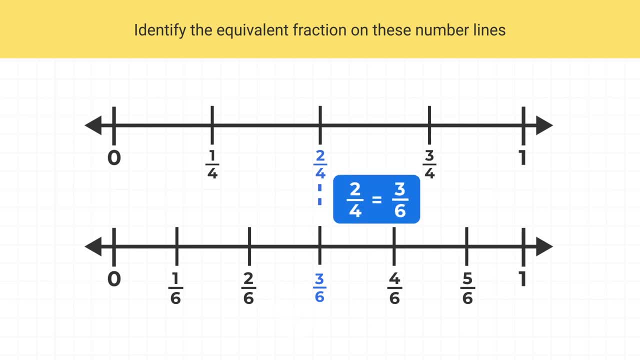 So two-fourths is equal to three-sixths. What about three-fourths? What fraction is at the same place as three-fourths? There's no fraction on these number lines on the same place as three-fourths. So the only equivalent fraction on these number lines is the two-fourths and three-sixths.